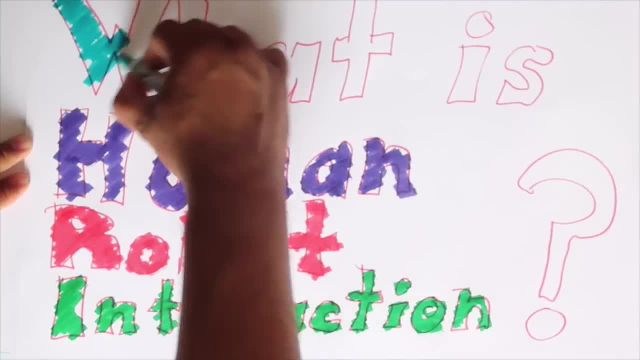 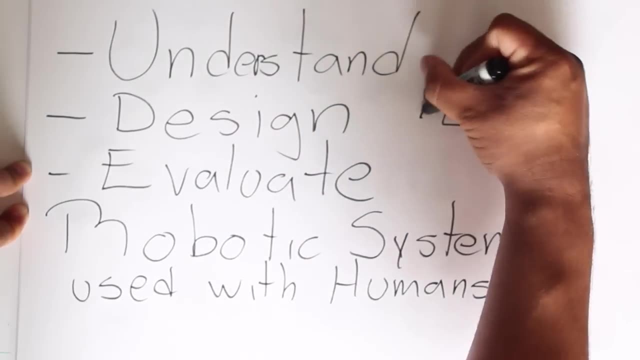 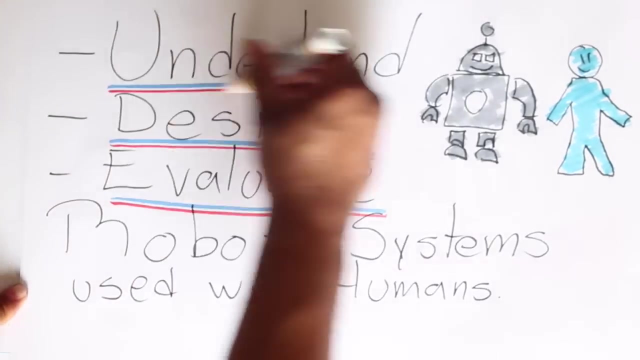 of the future eventually come true. But what is human-robot interaction? According to Micheal Goodrich and Alan Schultz, human-robot interaction is a field of study dedicated to understanding, designing and evaluating robotic systems for use by humans. Human-robot interaction is a multidisciplinary area of research comprising research in robotics. 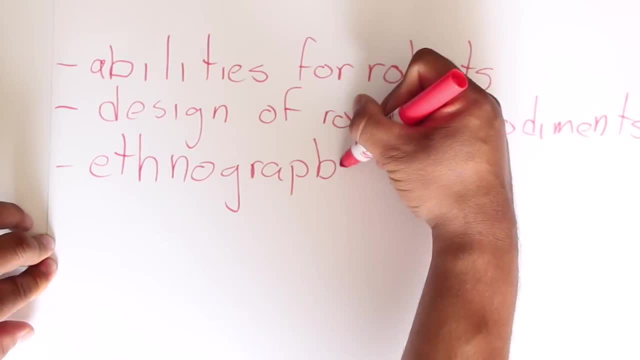 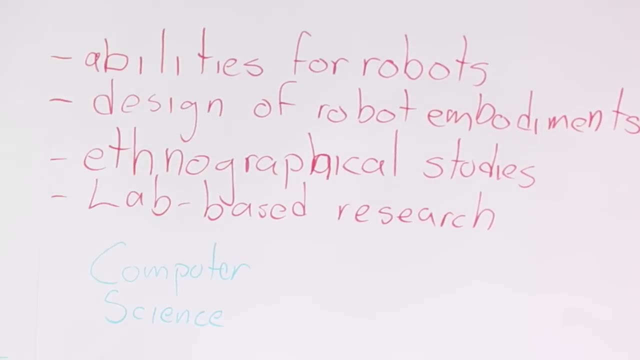 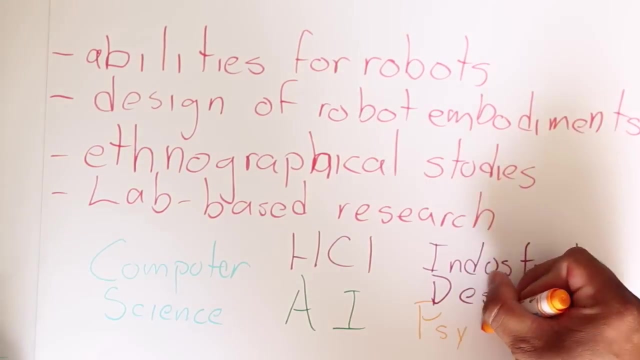 comprising of the technological abilities of robots, the design of robot embodiments, ethnographical studies on robots and lab-based research, where human participants interact with robots in a controlled environment. Therefore, the disciplines involved with human-robot interaction are computer science, human-computer. 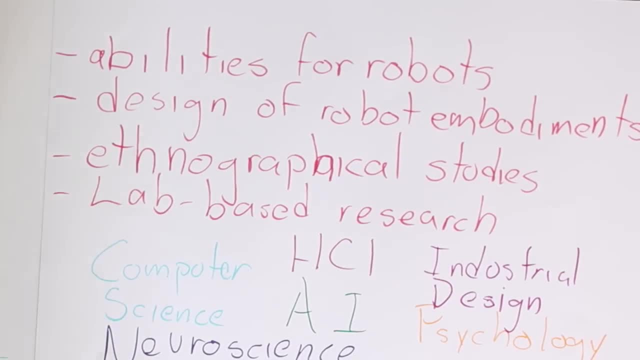 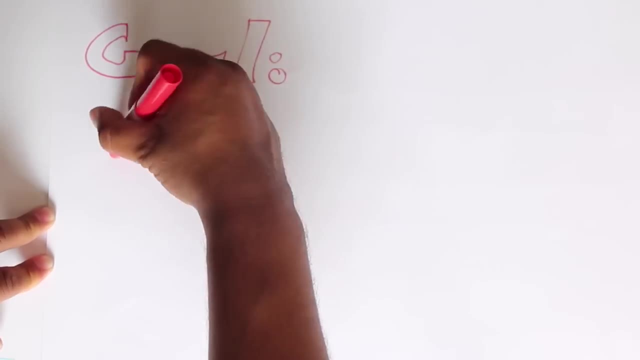 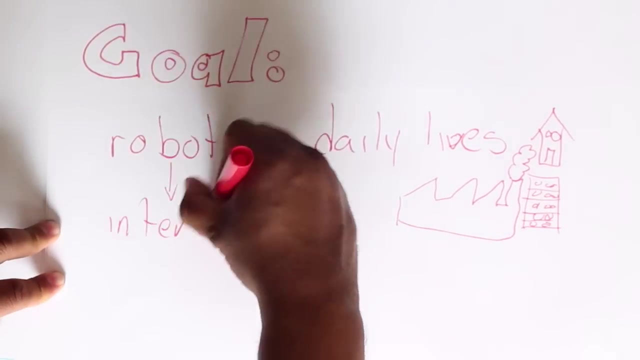 interaction, artificial intelligence, design, psychology, neuroscience, machine learning and many more. The goal of most human-robot interaction research is to promote the uptake of robots in our daily lives across different environments. That means in the future, humans will interact with robots as much as with other humans. 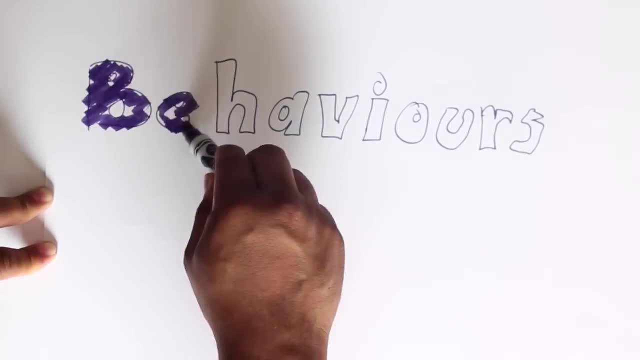 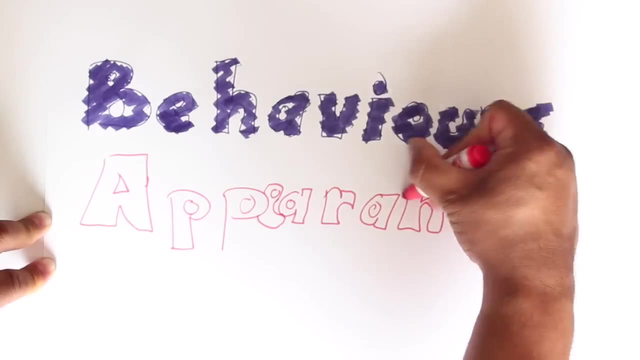 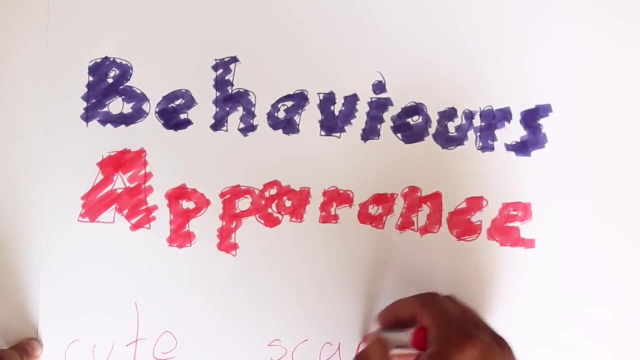 This extent of social interaction gives birth to many interesting problems that researchers are trying to solve. Human-robot interaction researchers mainly are investigating what are the optimal behaviors and appropriate physical appearance of the robots. There are different kinds of robots: Some are cute, others are scary and some are exact replicas of Japanese researchers. 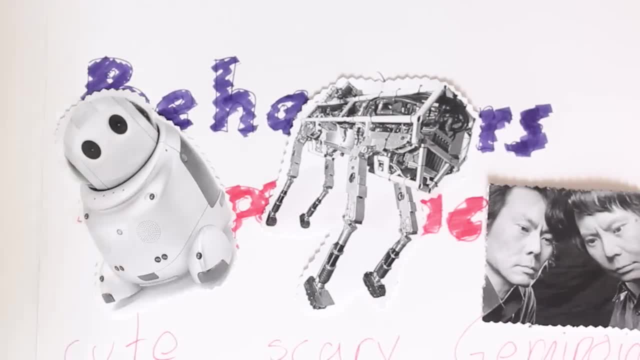 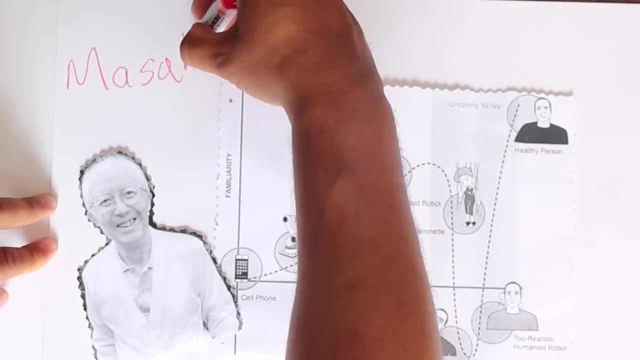 such as the Geminoid. So what should a robot look like and how must it behave? The Uncanny Valley provides us with some answers. In 1970, a Japanese scientist, Masahiro Mori, proposed a theoretical model linking robot. 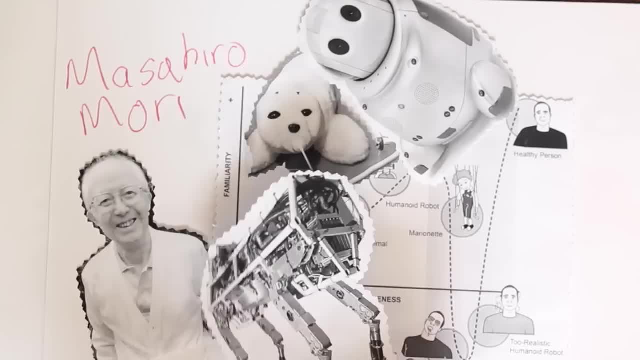 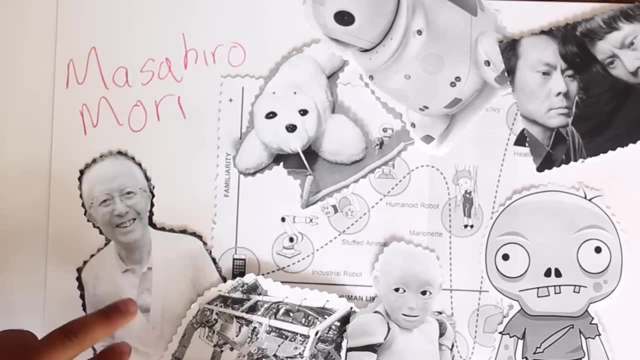 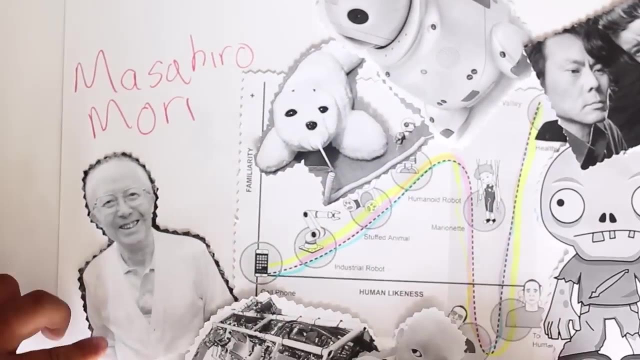 behavior with robot appearance. Mori suggested that robots that look and behave almost like humans have a tendency to cause aversion in humans. Think of a zombie. Many believe this revulsion is caused by a fear of death. The Uncanny Valley is primarily hypothetical and scientific evidence has both supported. 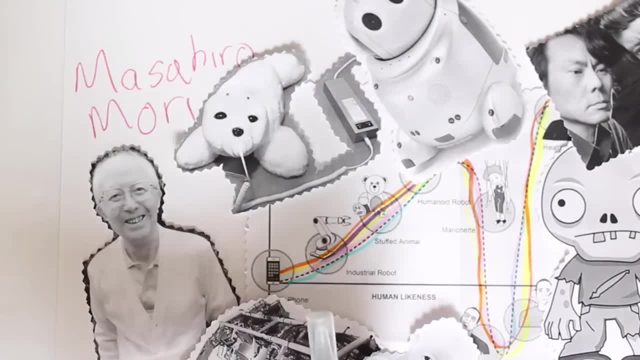 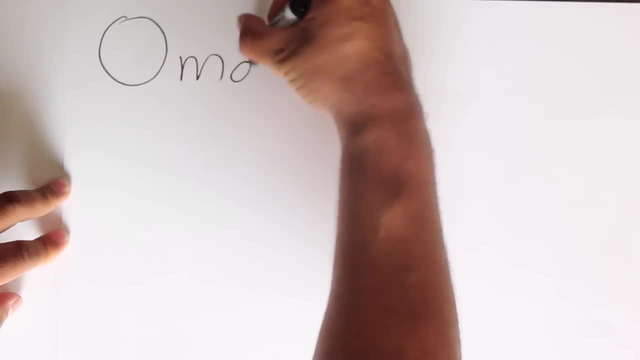 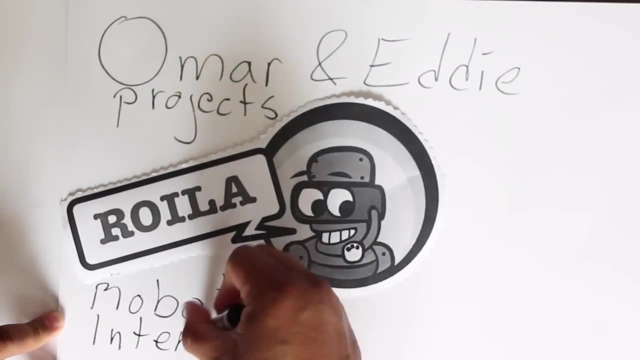 and negated it. However, it does provide a theoretical underpinning onto which human-robot interaction research can be built. We have been involved in exciting research projects within the area of human-robot interaction. We have created a language- ROILA stands for Robot Interaction Language.